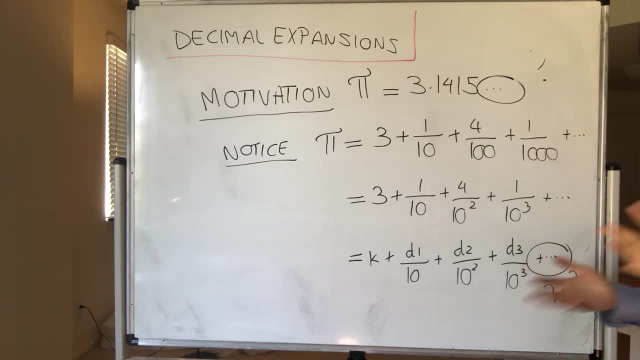 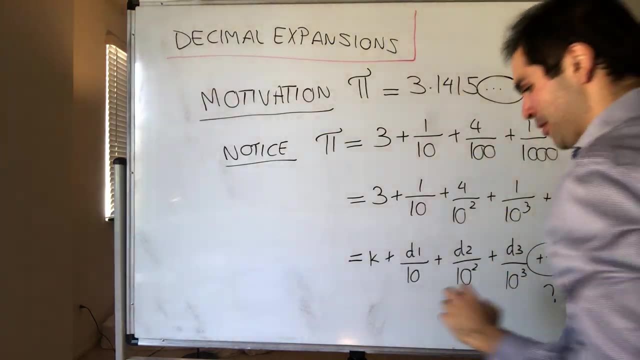 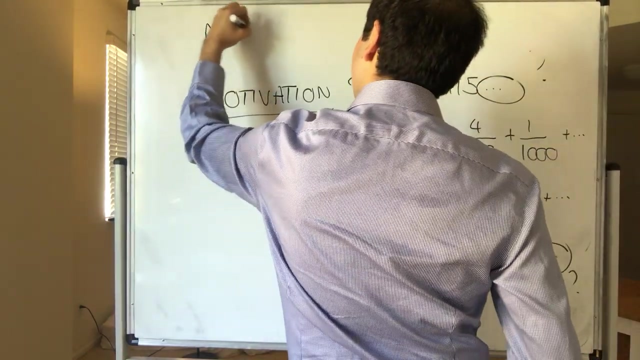 we don't know what the series is, We just know what a sequence is. But luckily we can actually define that more precisely, namely by just considering step by step terms, in some sense. So let'sors, what do we have? 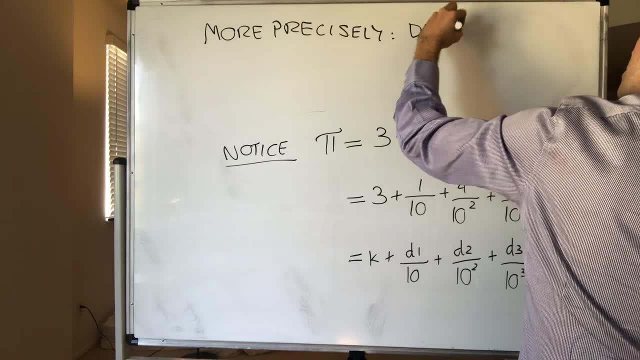 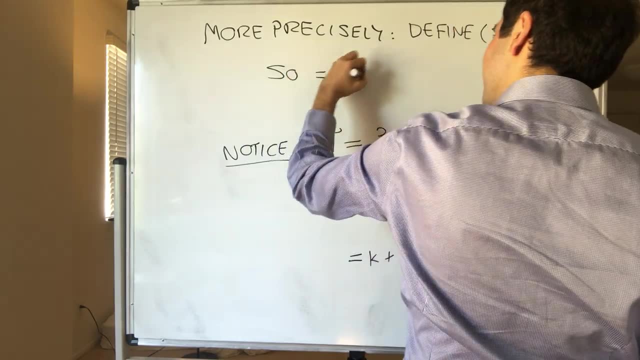 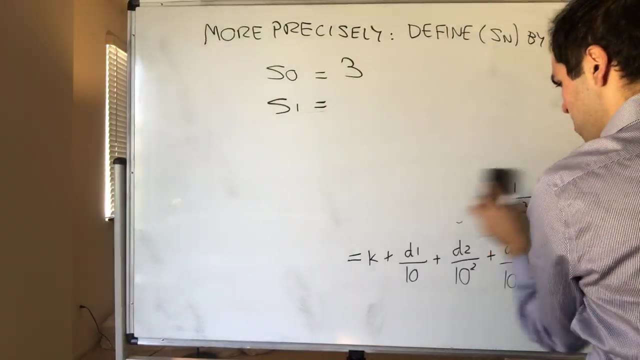 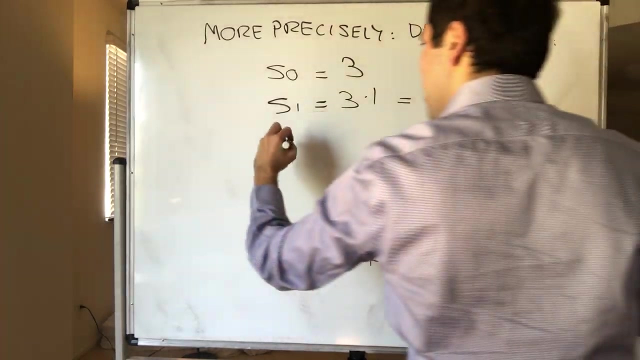 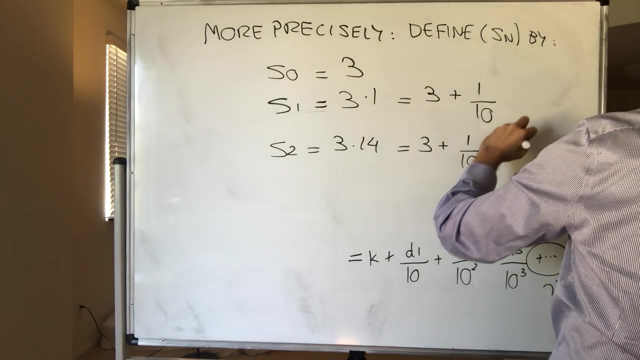 Well, we have defined the following sequence: Define Sn by the first term is just three, So Sn is three, which is k, and then s1 is 3.1.. which is again 3 plus 1 tenth. S2, it's 3.14, so 3 plus 1 tenth plus 4 over 10 squared. 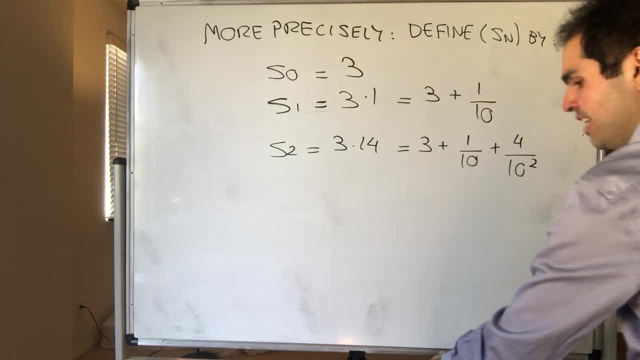 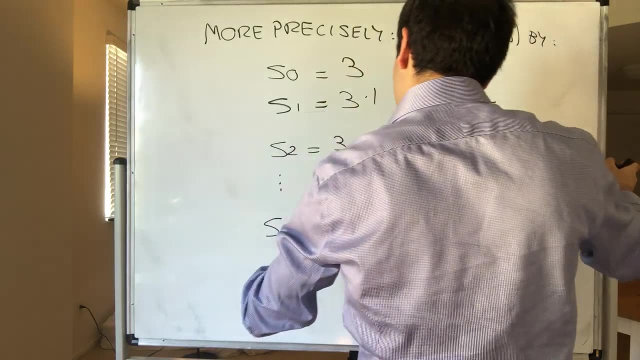 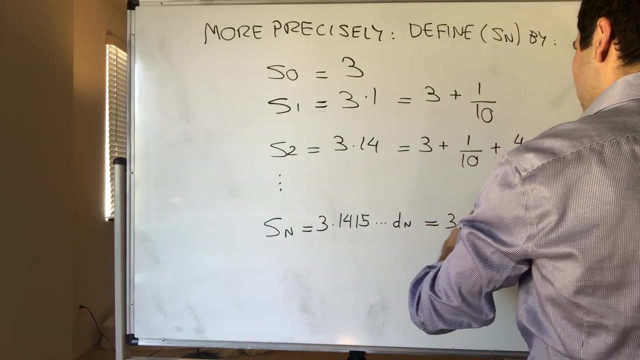 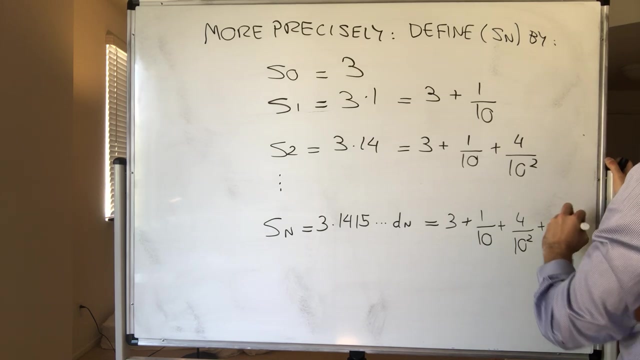 and more precisely Sn is up to the nth decimal place. So Sn is just 3.1415, dot, dot, dot up to dn. So that's 3 plus 1 tenth plus 4 over 10 squared plus a finite sum, so well-defined dn over 10 to the n. 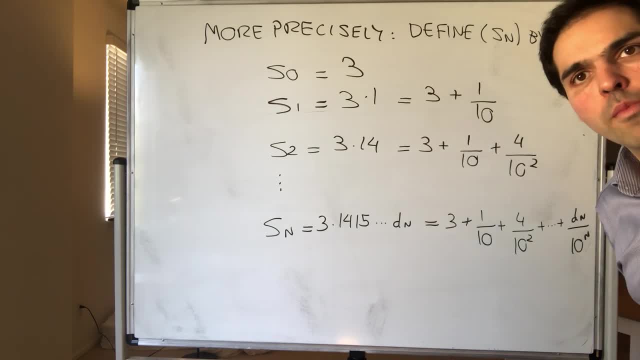 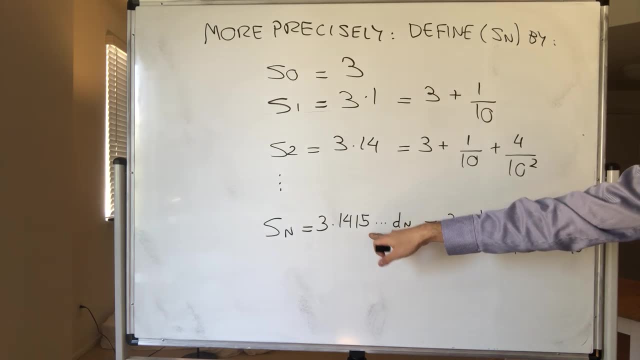 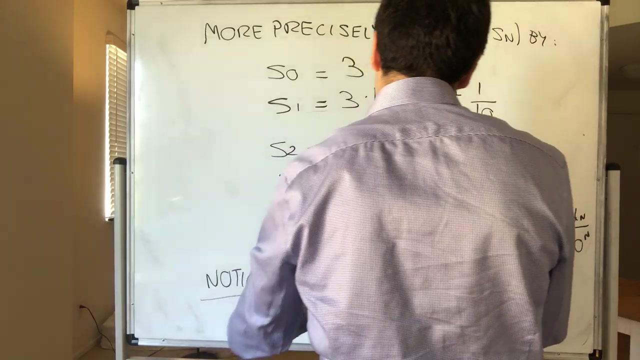 Now here's the thing: This sequence isn't just an arbitrary sequence, It has some very special properties. First of all, notice this sequence is bounded above All those numbers. they're actually smaller than 4, and that's guaranteed. So notice, not only Sn is bounded above. 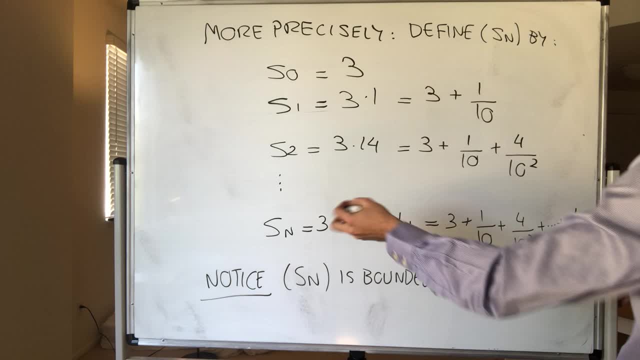 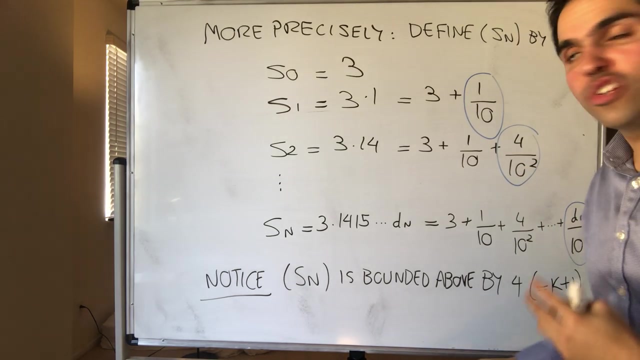 in this case by 4, but 4, it's really 3 plus 1, so in general it's k plus 1.. And not only that, notice: at each step we're adding positive terms, So actually this sequence is increasing. So this 3.1 is bigger than 3,, 3.14 is bigger than 3.1,. 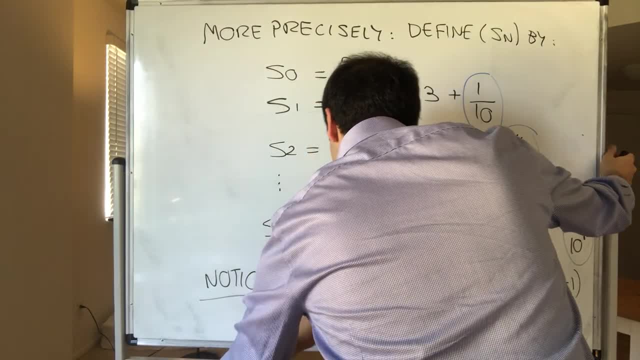 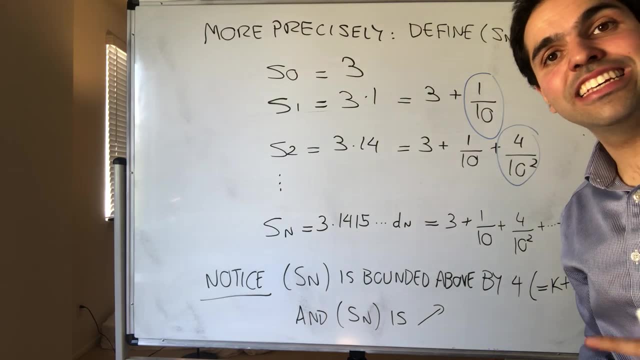 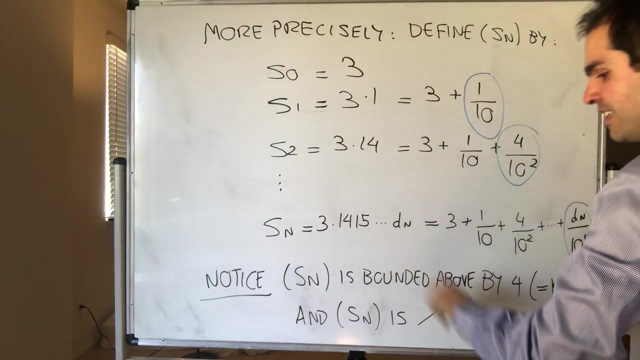 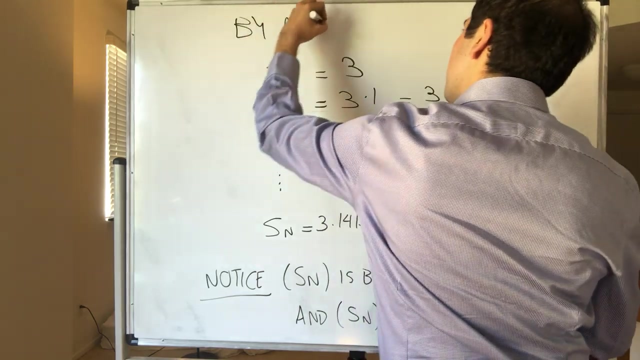 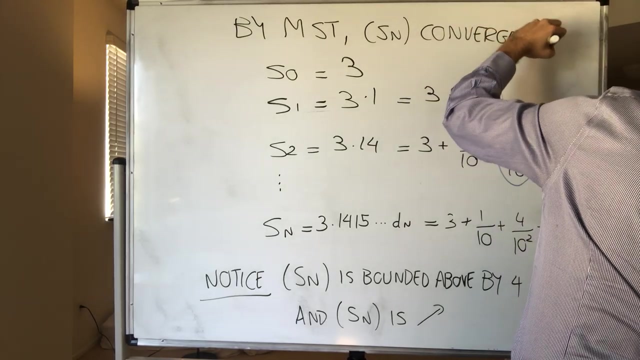 so actually, Sn is also increasing. And what do we have? A bounded above sequence that's increasing. Bam. We can use the monotone sequence theorem. So we know this sequence is convergent. So bye, MST. monotone sequence theorem: Sn converges to S. and what is S? 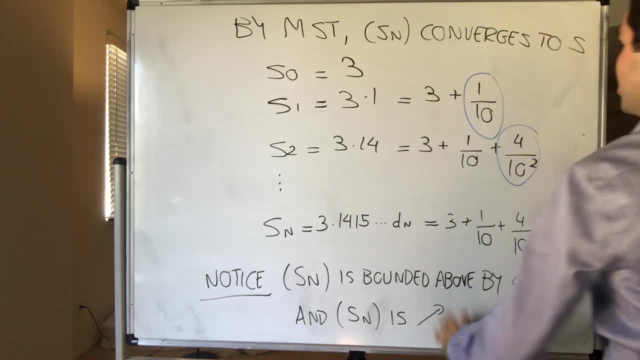 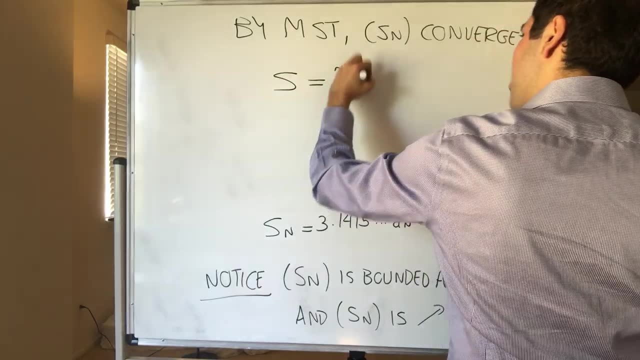 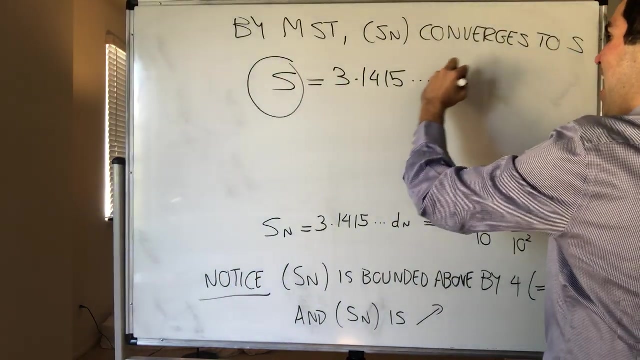 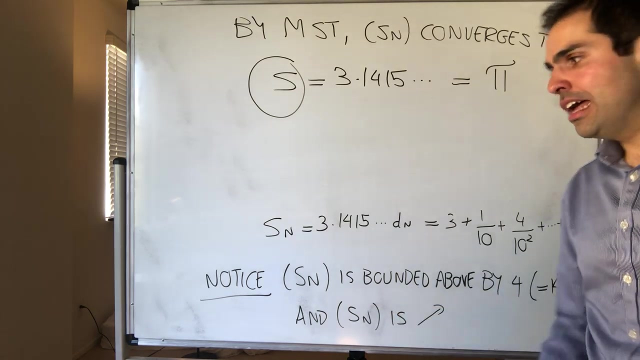 It's really just this infinite decimal expansion, S, which is again really symbolic. It's 3.1415, but it's precisely this limit that we call pi. So, in other words, what is a real number? It's just a limit of decimal expansions. 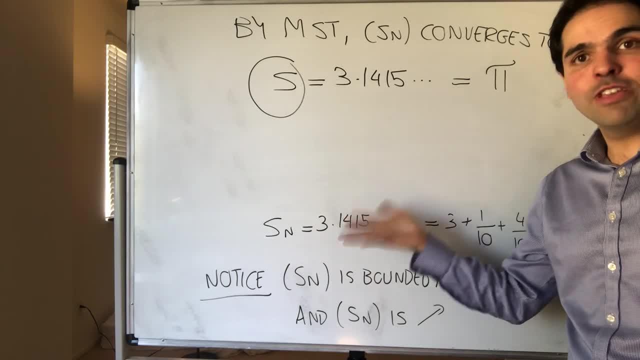 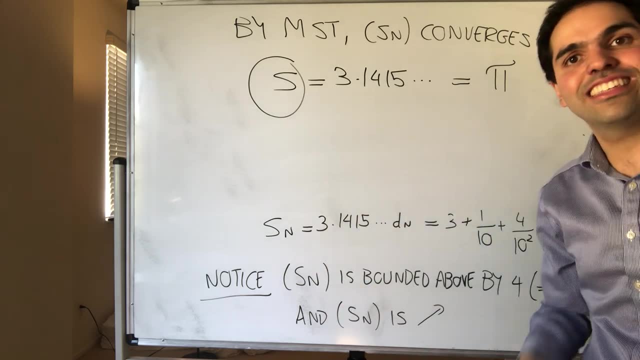 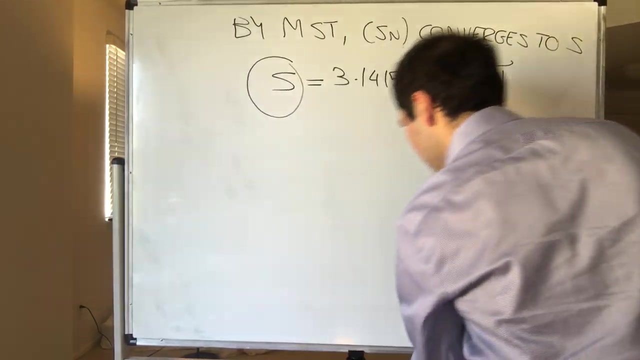 And again, that's really what you think of in your mind: 3.1415 dot dot dot. but it's really the dot dot dot dot. It's just a result of taking successive increasing sequences. So definition: Stephen R. 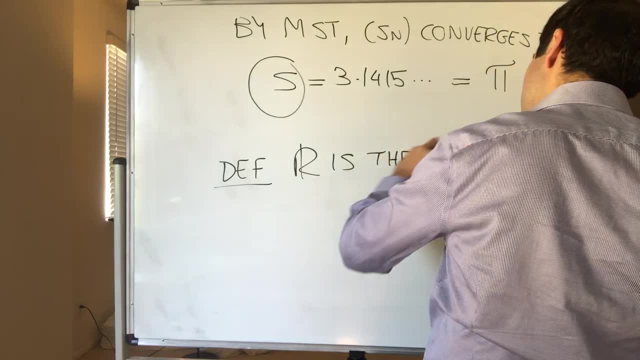 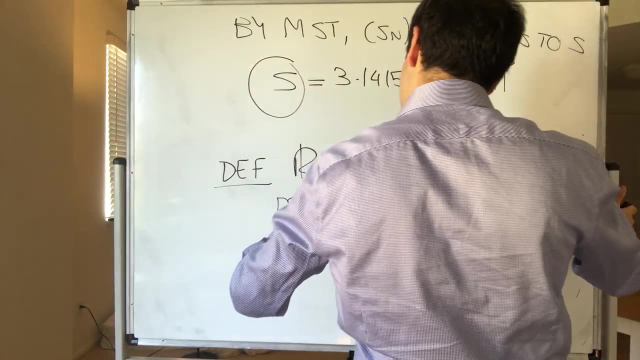 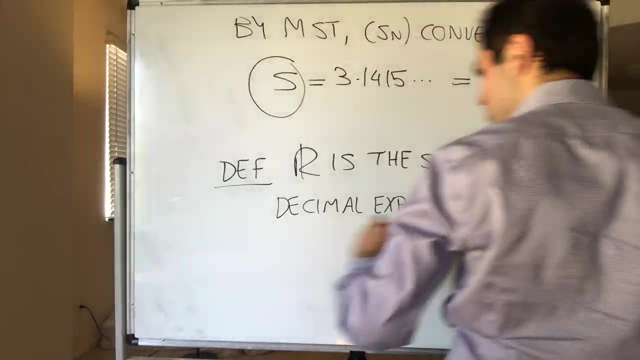 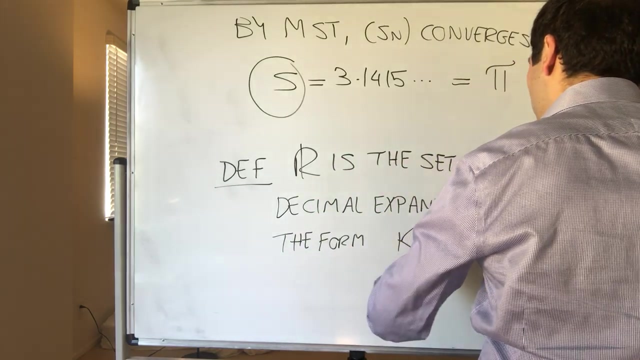 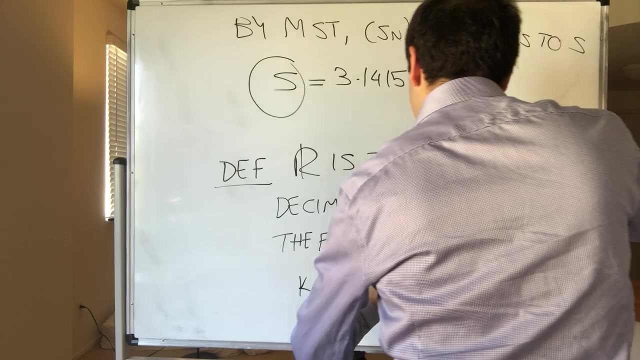 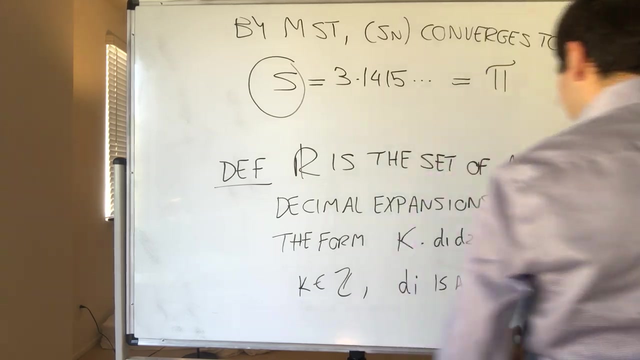 R is just the set of all those limits, so all decimal expansions of the four, again k, dot, dy, d1, d2, d3, etc, etc, where k is an integer and then each di is a digit between 0 and 9.. 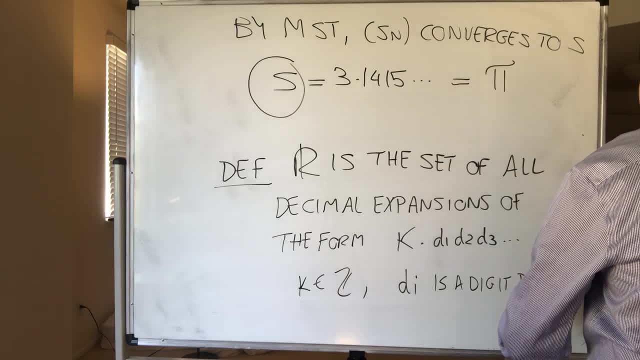 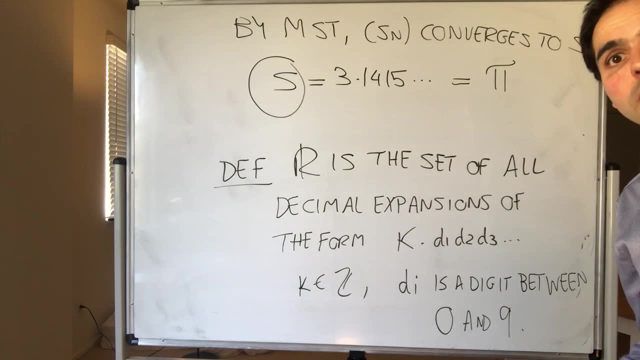 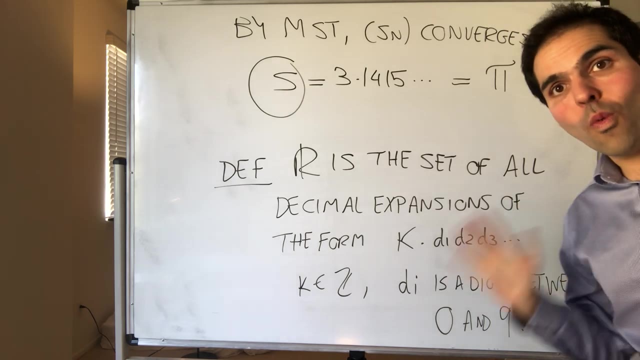 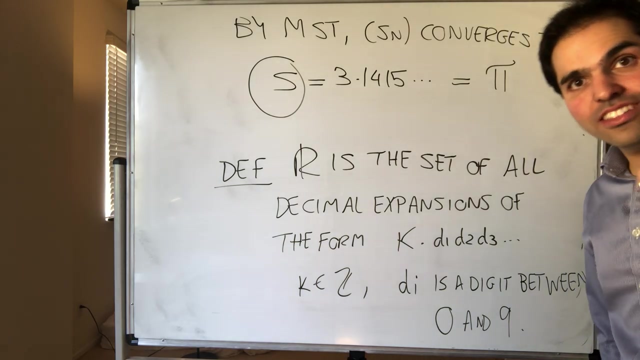 So, again, this is a very natural definition, which is again the one you've been acquainted with. However, there are many problems with this definition and there's really a reason why we usually define real numbers with Vatican cuts. In fact, there's a reason why we usually define: 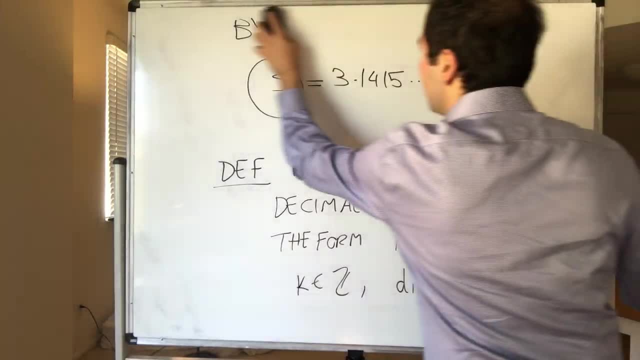 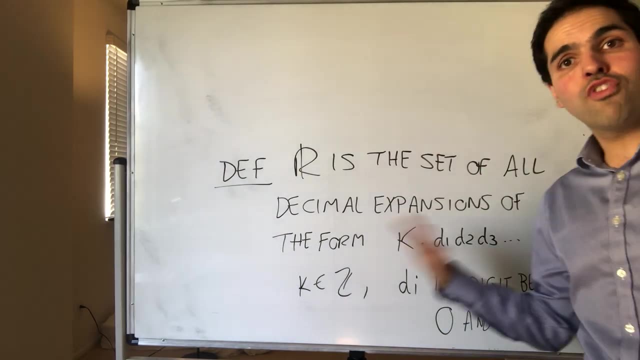 real numbers with Vatican cuts. In fact, there's a reason why we usually define real numbers with instead of this one, because look okay, real numbers are just decimal expansions. but then how would you know, for instance, if square root of 2 even has a decimal expansion? Remember square. 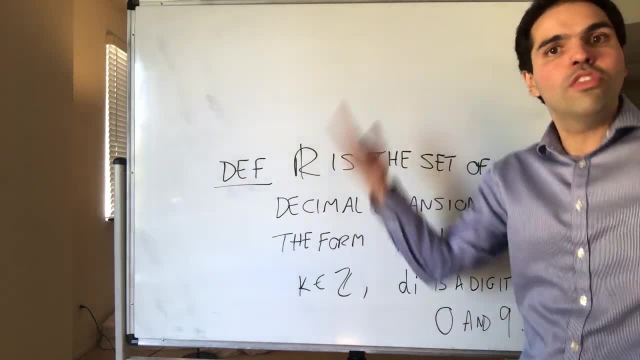 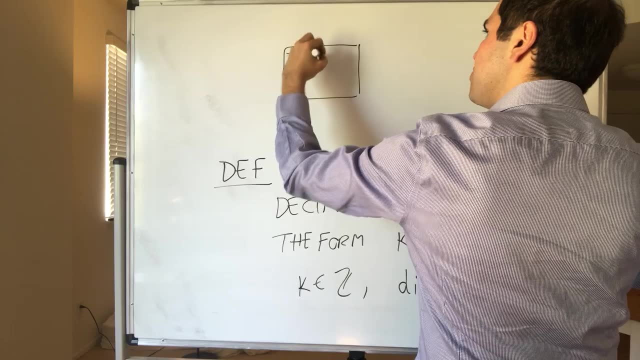 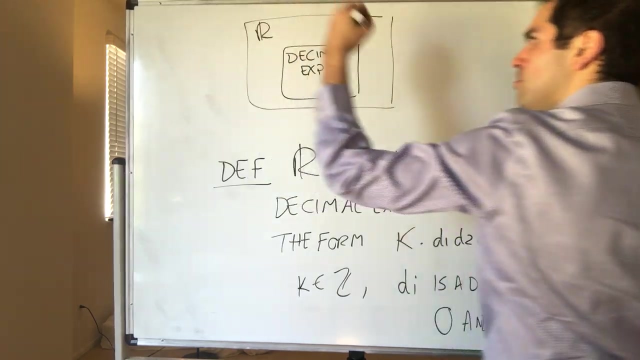 root of 2 is this number, whose square is 2.. How would you know that number has a decimal expansion. So, in theory, what could happen? you could have that the decimal expansions do not cover all the real numbers that we know, So there could be a real number without the decimal. 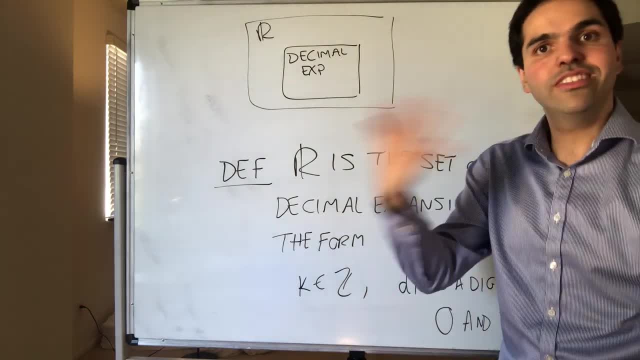 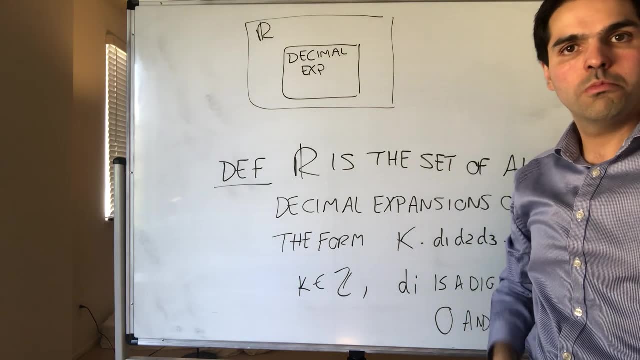 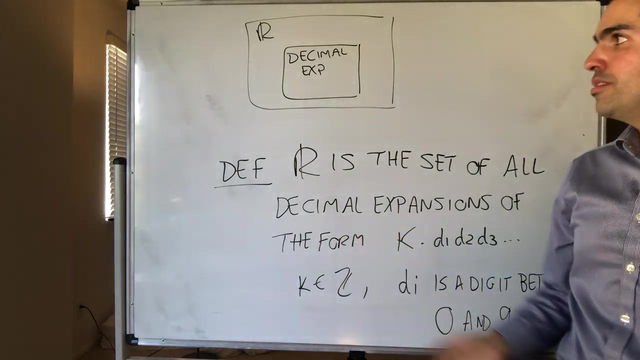 expansion. However, one can prove in section 16, which I won't cover, unfortunately- that indeed every real number has a decimal expansion. Here's another issue: How can we distinguish rational numbers with real numbers? You see, in other words, what special decimal expansion does. 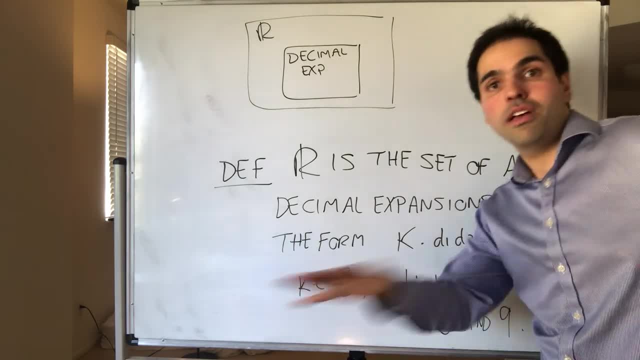 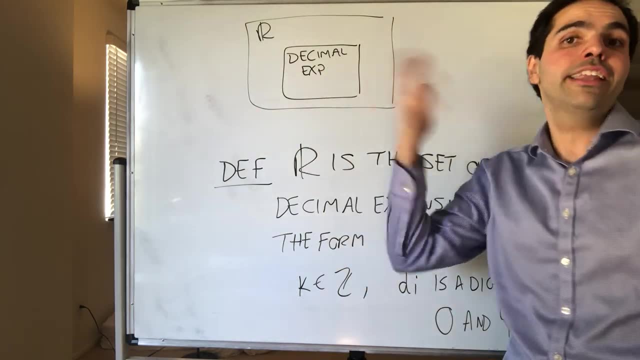 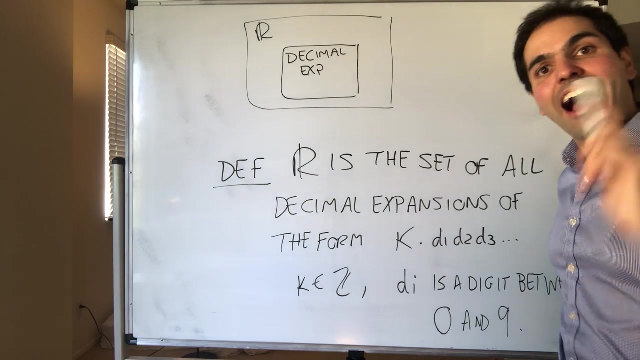 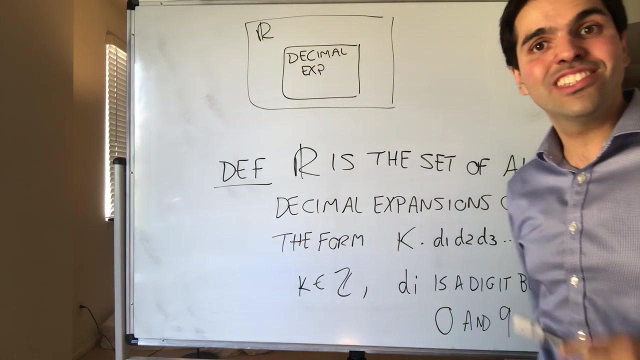 a rational number have, And again, at this point we don't really know. Later, if you're interested, we can show that rational numbers have periodic decimal expansions. And not only that, the biggest problem, how can we show, using only this definition, that the real numbers satisfy the least upper bound property? 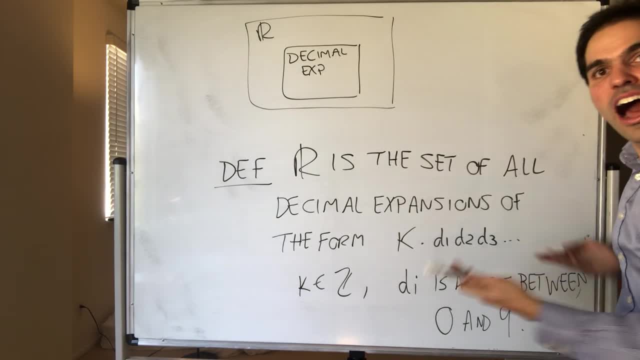 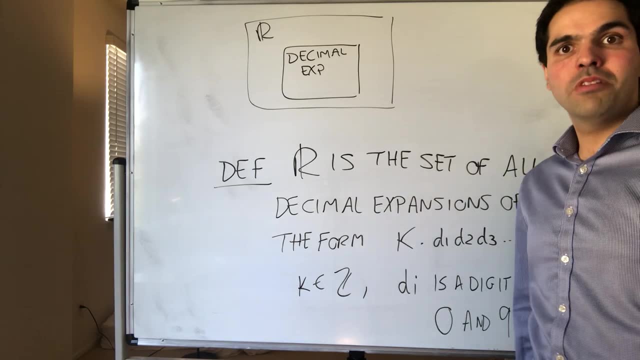 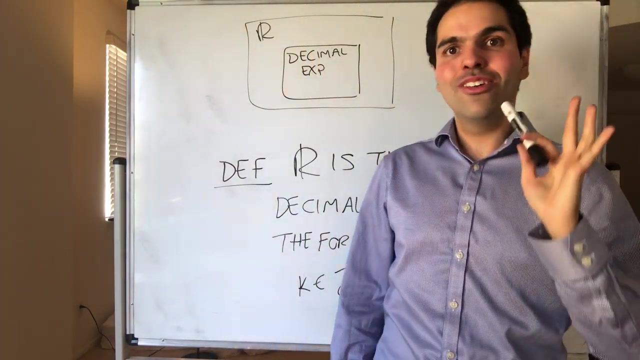 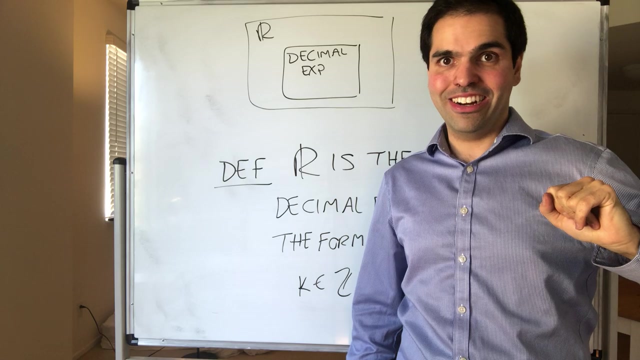 Suppose I tell you real numbers are those expansions, How do we know that every non-empty set that's bounded above has a least upper bound? Good luck proving that. So you see, the thing is delicate cuts. I know they look very ugly and don't judge them. they have their own beauty, but they might look very ugly. 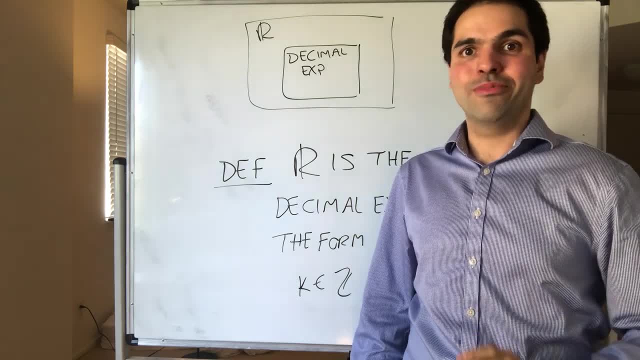 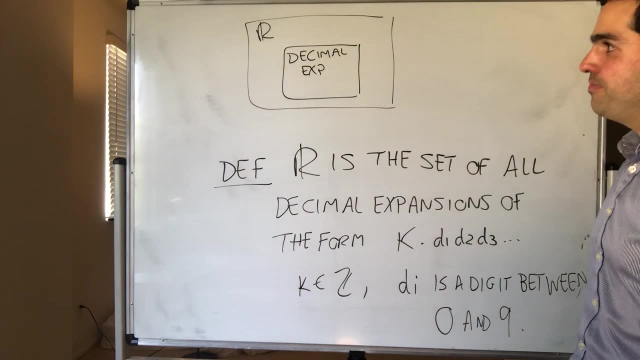 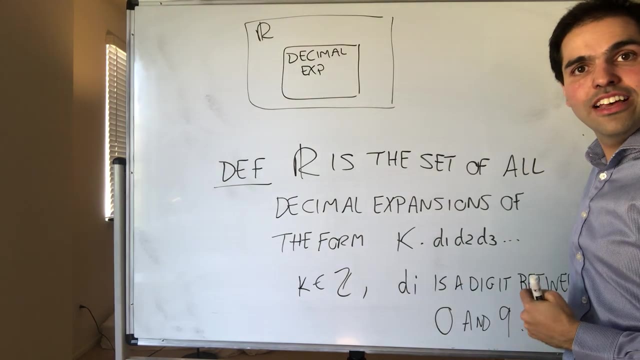 But they make proving least upper bound properties very elegant. So you see, that's why I tortured you with that, With that other definition. And not only that, there is another issue, because it turns out not only is this definition bad, it's also flawed. 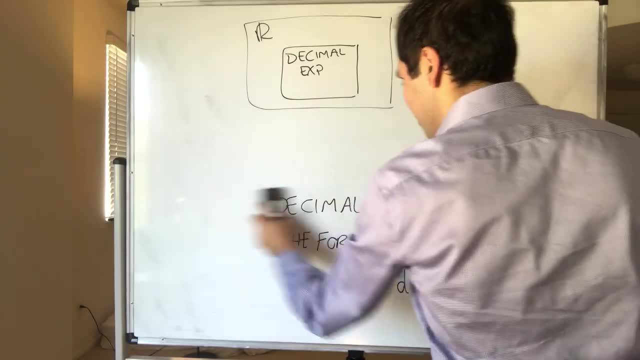 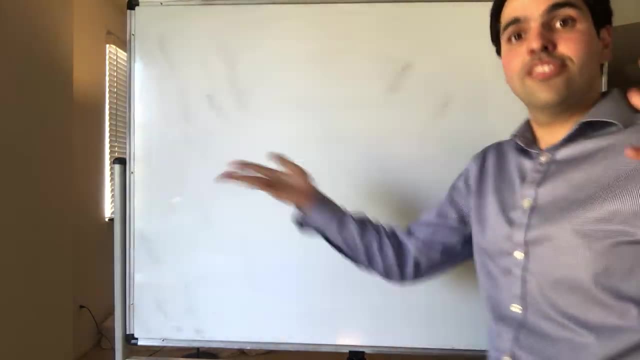 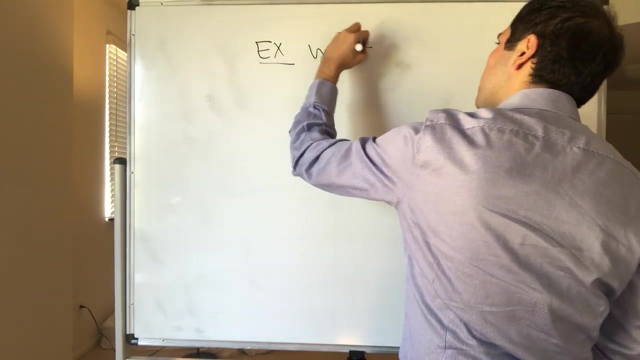 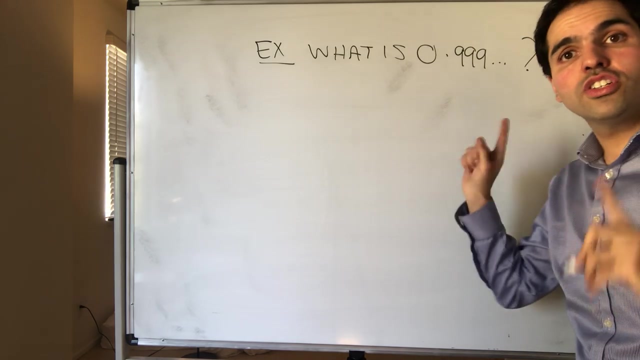 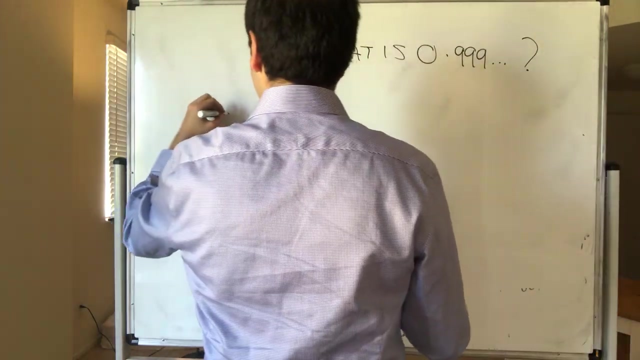 Because let me illustrate the following scenario: What you would like in theory is that two different decimal expansions should give you two different numbers. But look at the following: What is 0.99999.. And for this we need just a little result from geometric series, which is in your book, but also may know it from calculus. 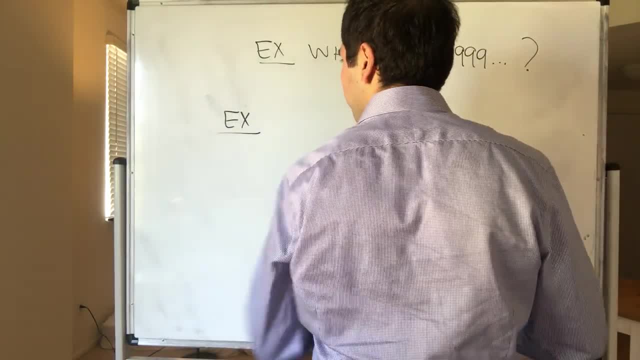 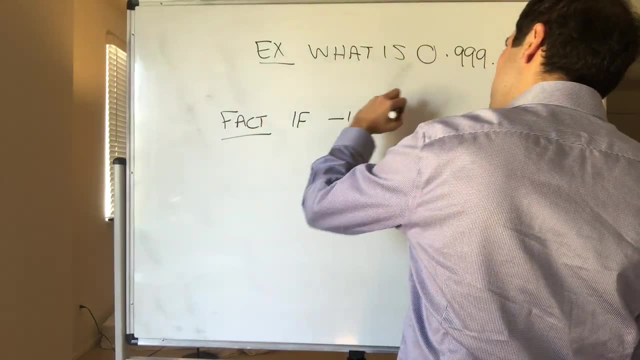 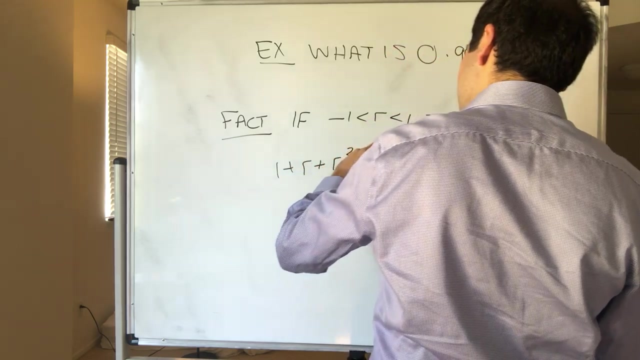 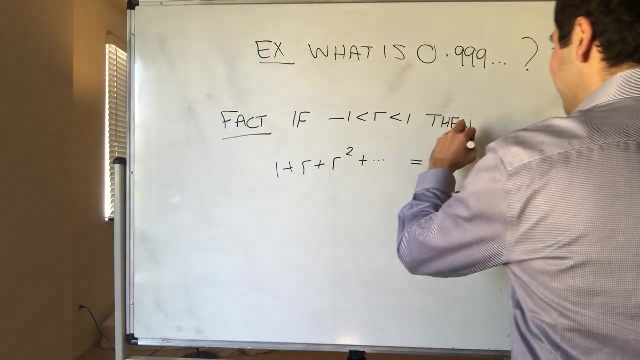 So fact, not example. If r is between minus 1 and 1, then 1 plus r plus r, squared plus dot dot dot. So the limit of those partial sums of those sequences is actually 1 over 1 minus r. 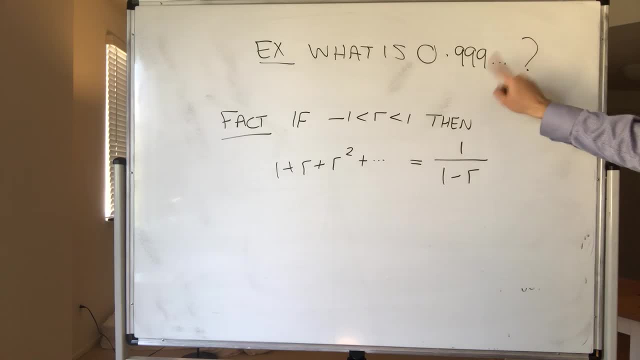 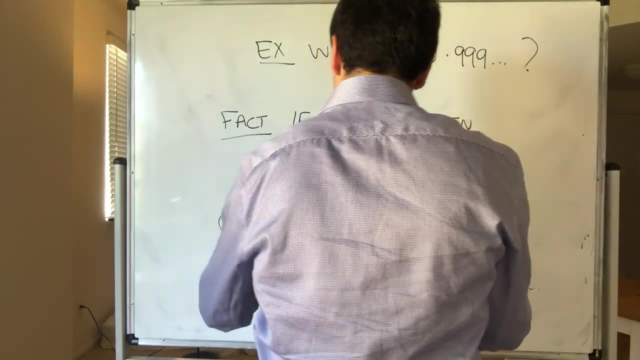 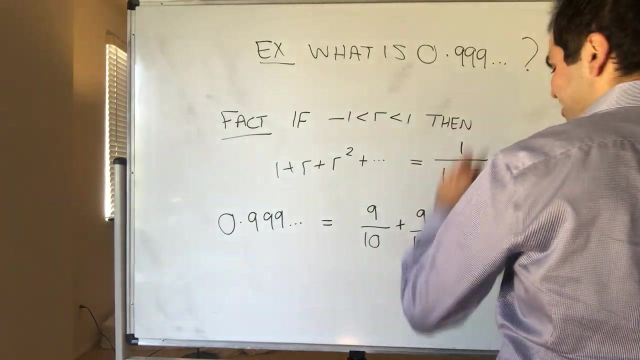 And again, You can show this. but, more importantly, how do we apply this to this example? Well, 0.999.. Well, by definition, that's just 9 tenths plus 9 over 100.. Plus not 9 thousand, but 9 over 1000. 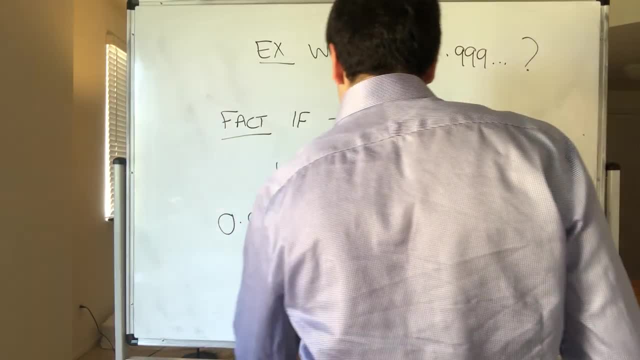 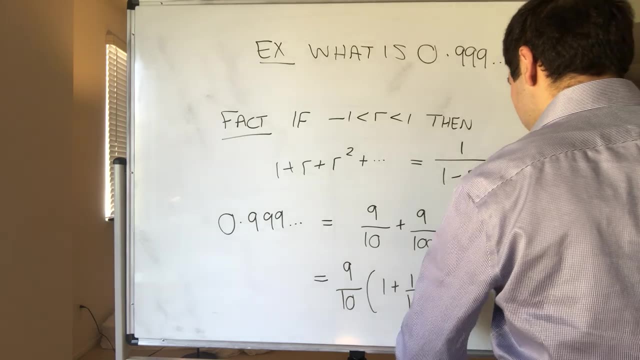 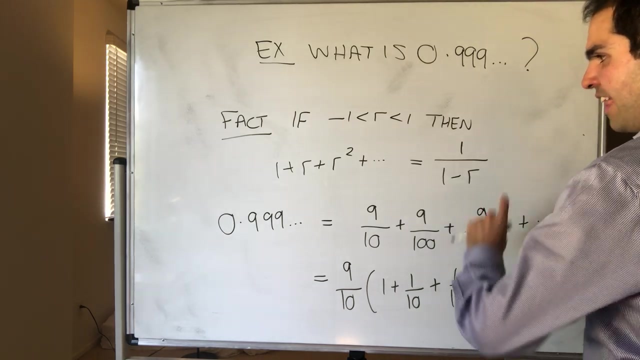 Plus dot dot dot, And really what this is is 9 tenths times 1 plus 1 tenth plus 1 hundredth plus dot dot dot, And it's really 1 plus 1 tenth plus 1 tenth squared, plus 1 tenth to the third power. 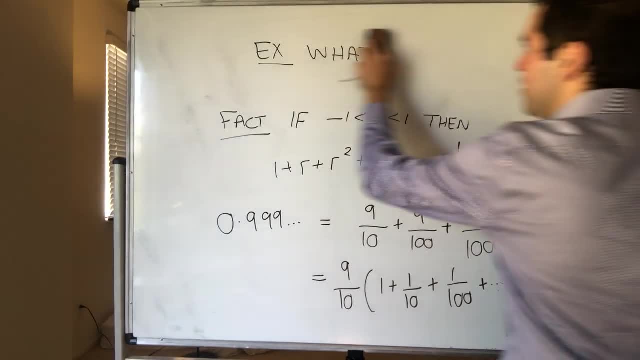 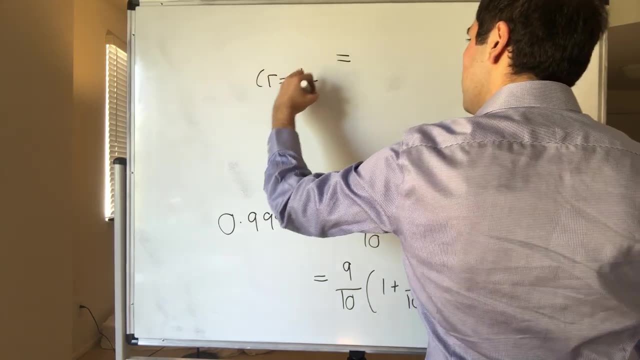 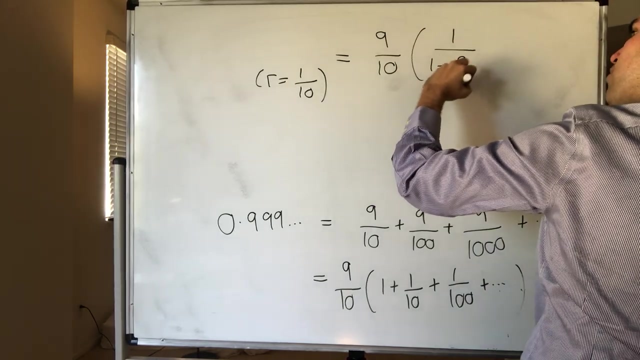 So it's really this thing, but with r equals 1 tenth, So it equals to again: r is 1 tenth. So again this factor 9 over 10 over 1 over 1 minus 1 over 10.. 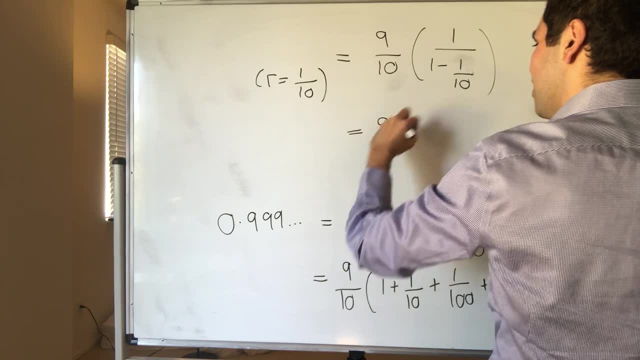 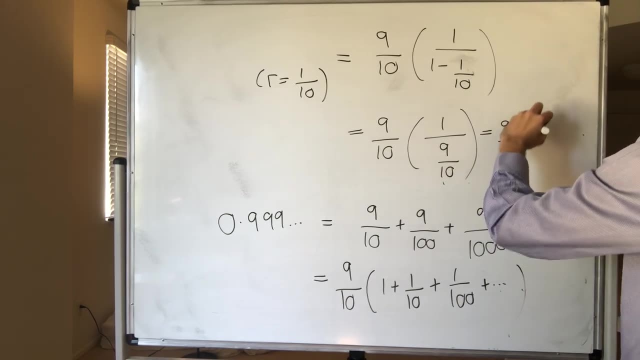 Because, again, that's the factor here, And so it's 9 tenths over 1 over 9 tenths, And really that's 9 tenths times 10 over 9.. Boom, boom, boom boom. 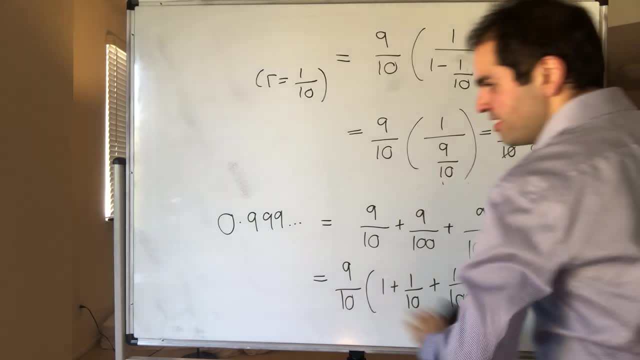 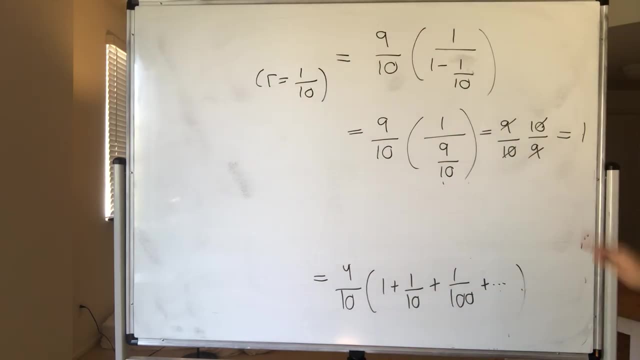 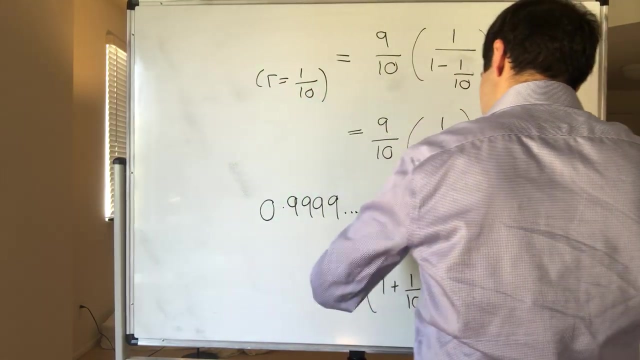 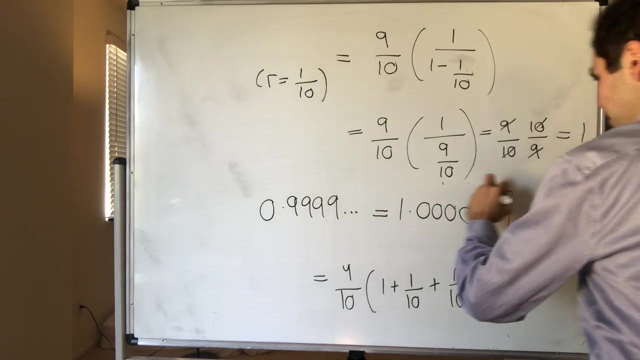 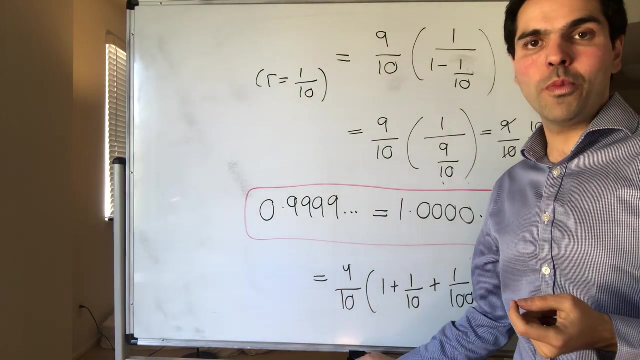 And that's 1.. In other words, this number 0.99999,, it's almost German 99999,, it becomes 1.0000.. So in fact, Notice, two different decimal expansions may give rise to the same real number. 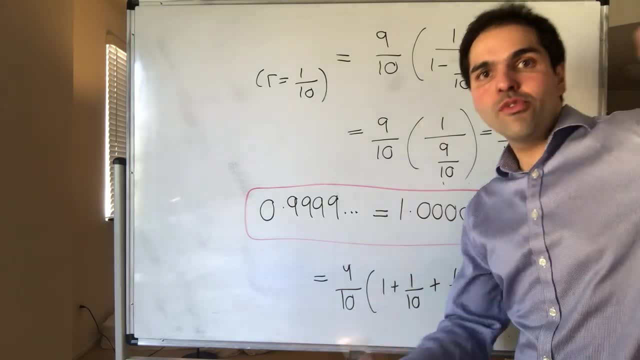 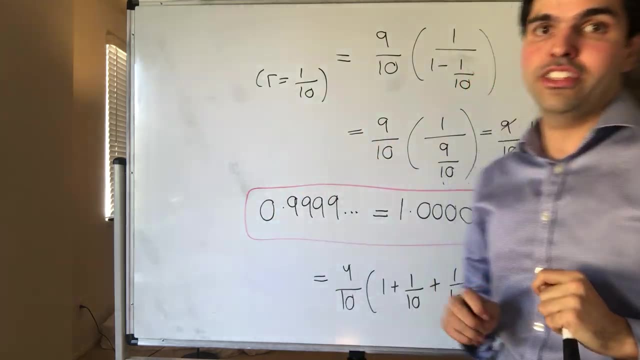 Which, again, ideally, we do not want to have. We would like that different expansions give you different real numbers, And in fact that was true for cuts: Different cuts give you different real numbers. And, however, last thing I want to say: 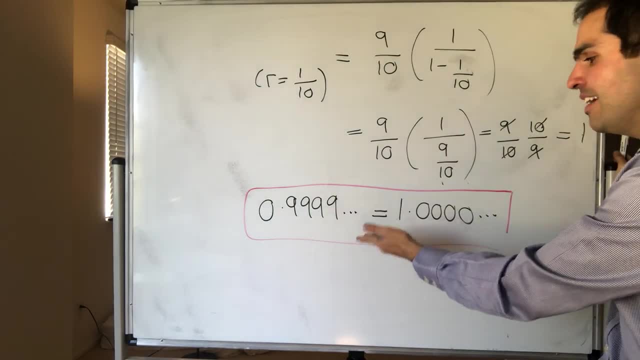 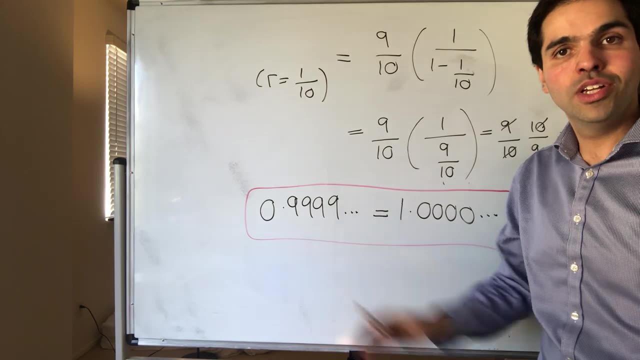 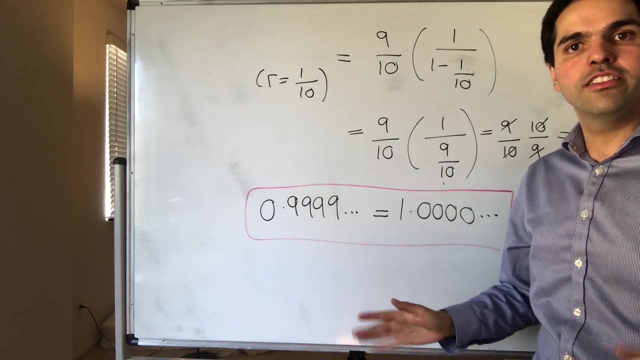 There is a way to get around this. Simply say that Throw away all the decimal expansions that terminate into an infinite string of 9s. So define the real numbers to be all the decimal expansions, Again, where di is a digit between 0 and 9.. 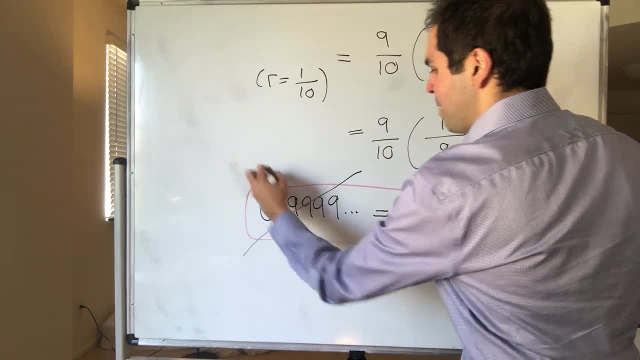 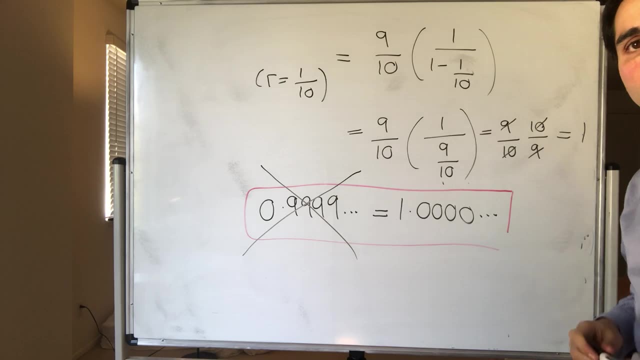 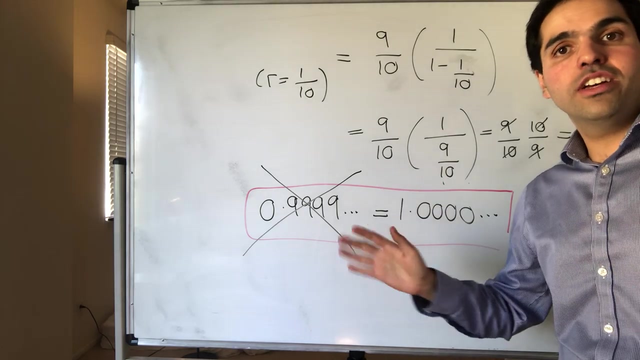 But ignore all the decimal expansions that end with a bunch of 9s. So in this case we would throw away this number, But just leave 1.000.. And in that way We actually have that Every decimal expansion gives rise to exactly one real number. 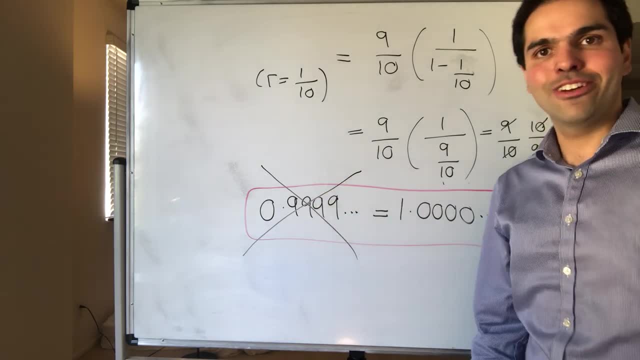 One-to-one way in some sense Alright. thank you very much. 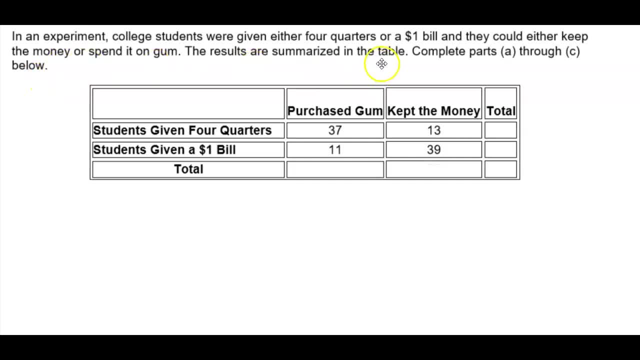 In an experiment, college students were given either four quarters or a dollar bill and they could either keep the money or spend it on gum. The results are summarized in a table and we're going to complete parts a through c below. So the first column is all the students that purchased. 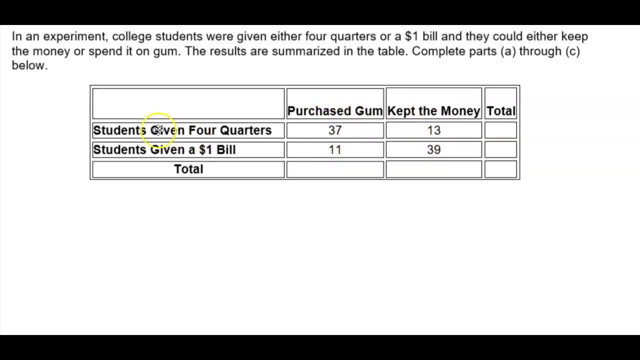 gum. The second column is that kept the money. The first row was the students that were given four quarters and the second row were students that were given a dollar bill. So let's take a look at the total for the students that were given four quarters: 37 plus 14 equals 50.. Students who